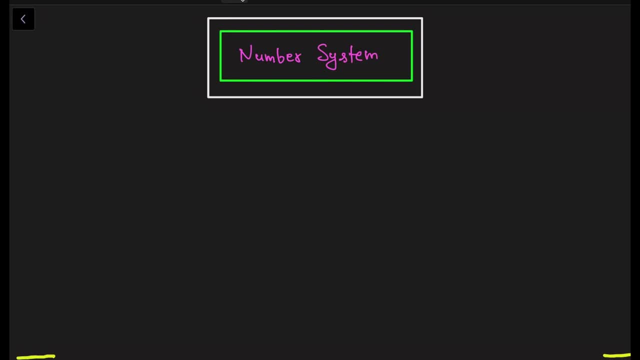 In that the modules related to set theory will be a very helpful lecture for them, And in this lecture we are going to discuss about number system. What is number system, What is the notation And which numbers come in it? Because our set theory depends on the number system. 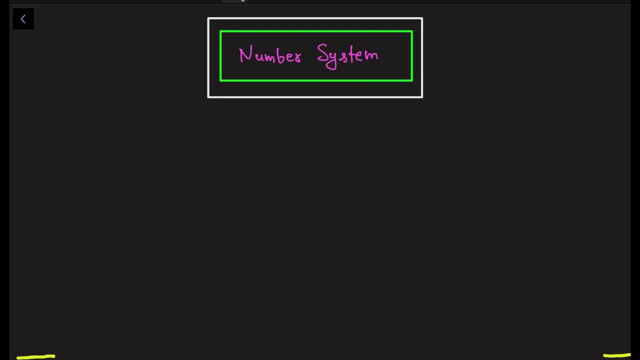 It is very useful When we will study algebra, in which we will study group theory, it will also be useful. It is also very useful in real analysis. So it will be very good for you to know the number system well. So let's start in the number system. 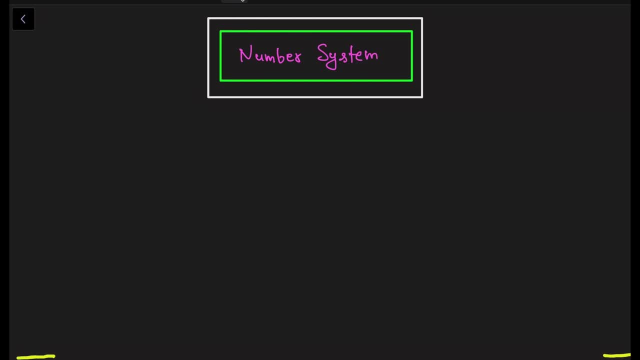 First of all, let's talk about the set of natural numbers. Let's talk about the number system. First of all, let's talk about the set of natural numbers, Natural numbers. If we talk about the set of natural numbers, then you all know that we denote this set with N. 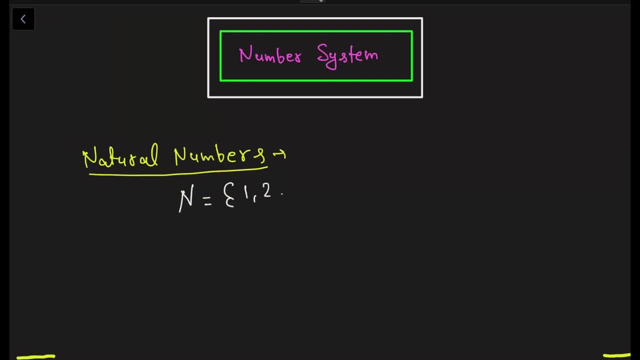 With capital N, And in this all the elements from 1,, 2,, 3 to infinite. all these come in the set of natural numbers. Its notation is denoted with capital N. Then, after the natural number, the set of whole numbers comes in it. 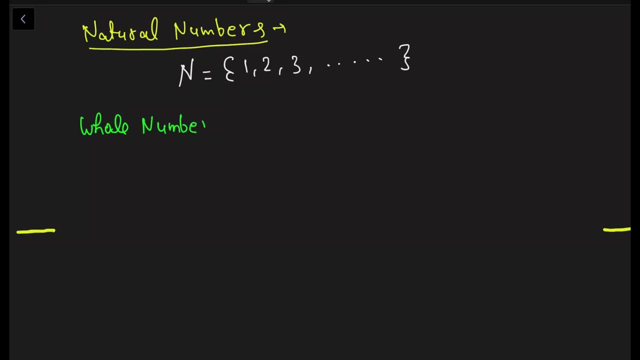 The set of whole numbers And the whole numbers. we also call them full numbers. Natural numbers are called natural numbers And in the set of natural numbers if we include one element, zero more, then the set of natural numbers becomes the set of whole numbers. 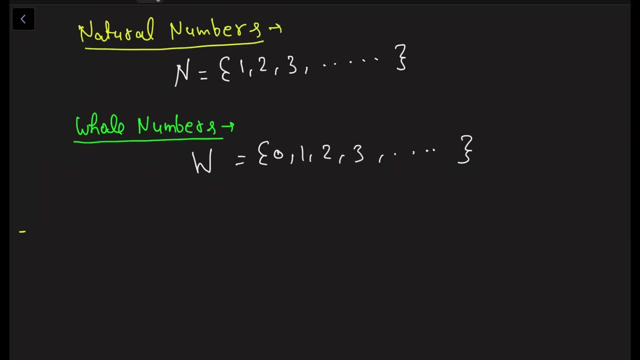 That is, it becomes a full number if we include zero in it. So our natural number is a natural number and the whole number is a full number. This is its notation. It is denoted with W. Then comes the set of integers. 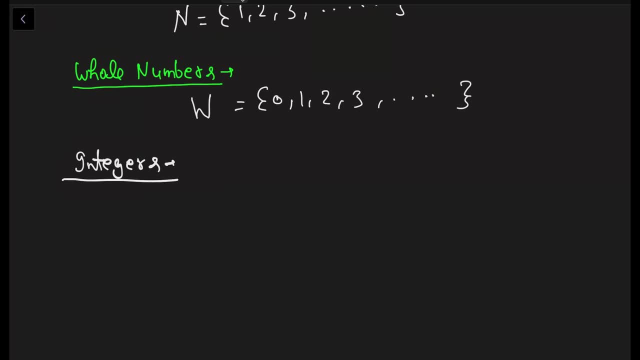 Integers. The notation of the set of integers is done in two ways. It is denoted with Z Or it is also denoted with capital I. What is the integer set? The whole number above you is 0,, 1,, 2,, 3,, dot, dot, dot, infinity. 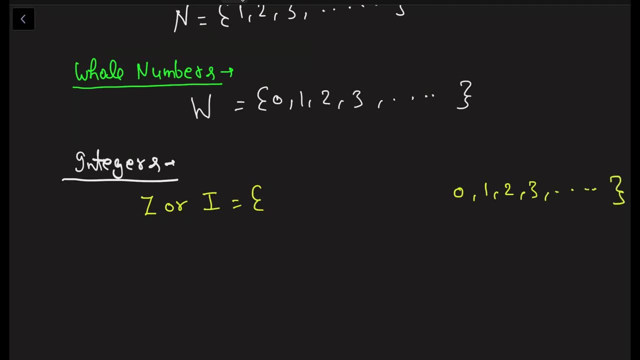 These are all our positive elements. There are non-negative numbers, And because you know that every thing has a negative, Then these numbers will also be negative, As if we take the negative of 1 here, Then the negative of 1 will be minus 1.. 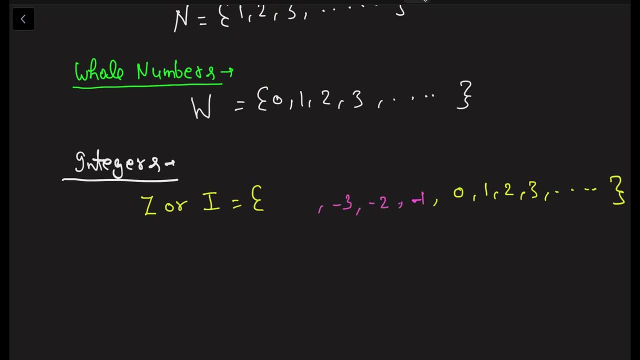 Then it will be minus 2.. Minus 3. And here it will go to your minus infinity. So all these numbers are called our integers. If you have negative elements and positive elements, And this zero neutral element is the middle number of the set. 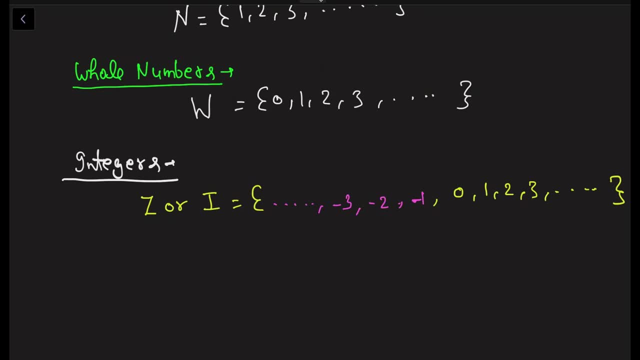 All this gives you the set of integers, And these elements here are called negative integers- I am writing this in short- And these are called positive integers. Positive integers, Okay, And if we include zero, The elements from zero to infinity are also called non-negative numbers. 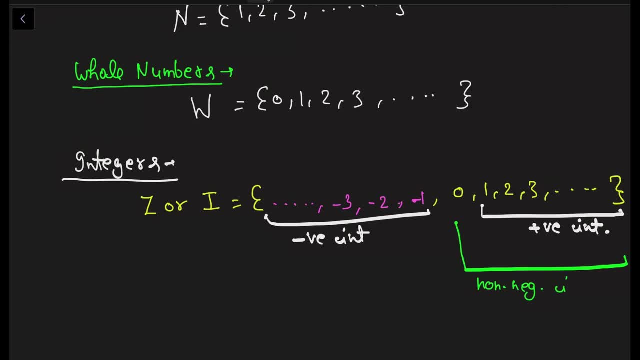 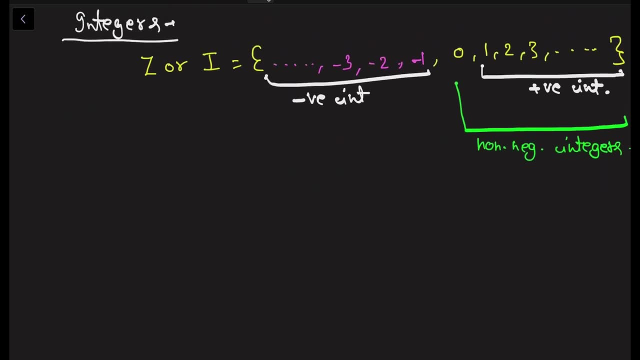 Non-negative integers. Non-negative integers. Okay, So this is our set of integers, In which positive and negative elements come. In this you will keep one thing in mind: That after zero, one will come. After one, two will come. 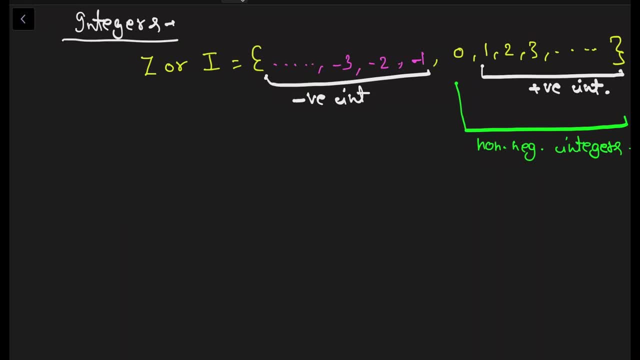 After two, three will come. Okay. Then, after this, our set is made, Which is called the set of rational numbers. Rational numbers, Now, what are rational numbers? There was a lack of fractional elements in this, So the fractional element was added. 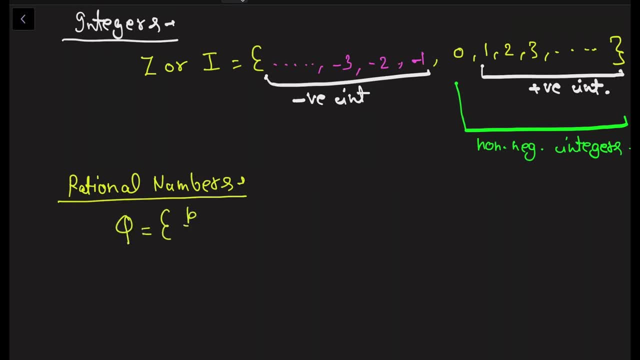 We denote the set of rational numbers with q, And in this there are elements of p upon q type. Okay, Where p and q both will belong to the set of integers z And this q element below will not be equal to zero. Okay, 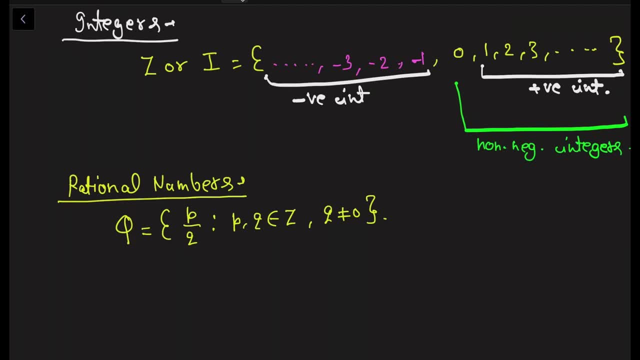 Because if it becomes zero, then we will get infinity, We will get an undefined number. So all the numbers in the form of p upon q, Where p and q can be the elements of our integers, Okay, And if our q is not zero? 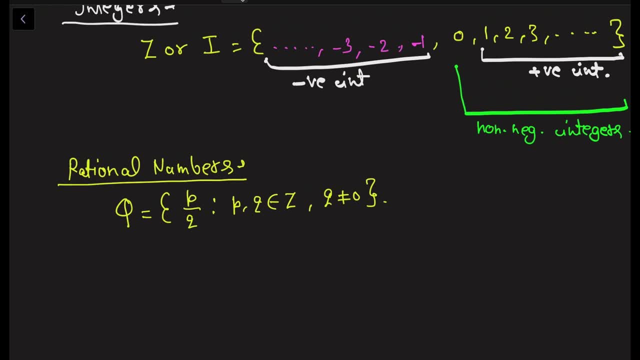 Then it will become the set of rational numbers. Now the thing is that all the elements of our integers are all negative and positive. Will we have rational numbers? Children get confused in this. I will tell you that they will all be rational numbers. 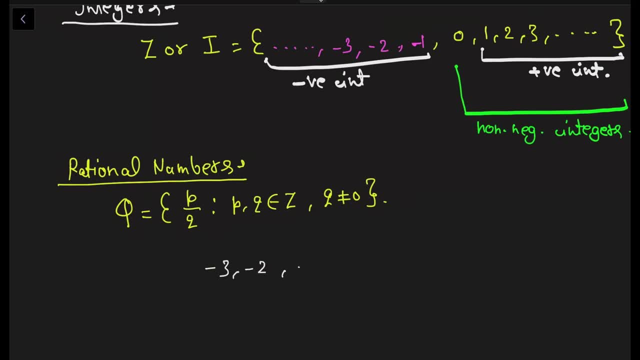 How? Because I have written the entire set of your integers here. Okay, If you see all the integers, that is, we will do the work of p And we consider q to be one. What do we consider q to be One? 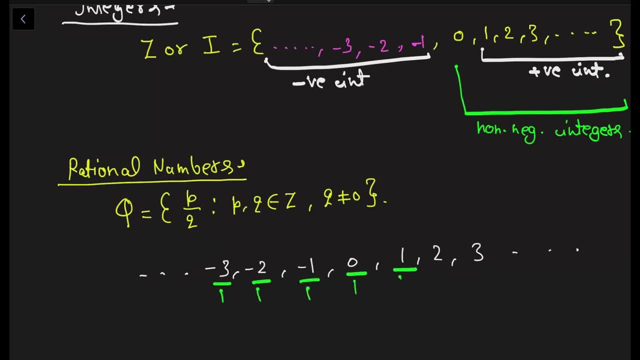 So if we divide all the integers by one, Then all these numbers will be converted into p upon q. Okay, And you can see that p and q both belong to the integer And the one below is not equal to zero. So that means all the integers are also rational numbers. 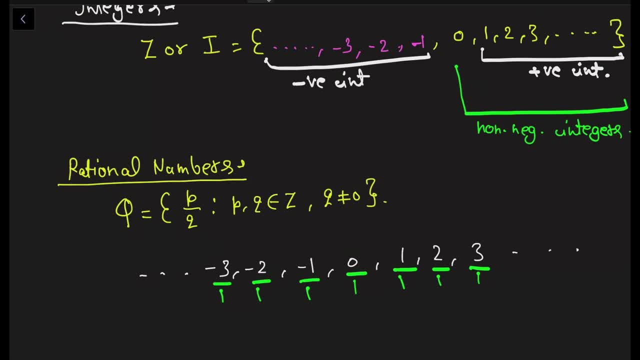 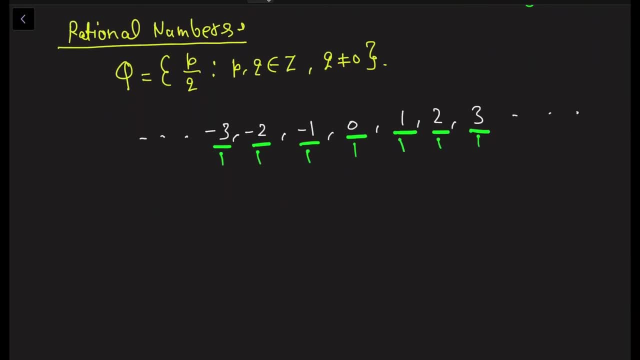 That means our integer set will become the subset of rational numbers. I will tell you this at the end. So all the integers are all our rational numbers. Okay, Now children get confused. Let's talk about the irrational numbers, IDIRATIONAL NUMBERS. 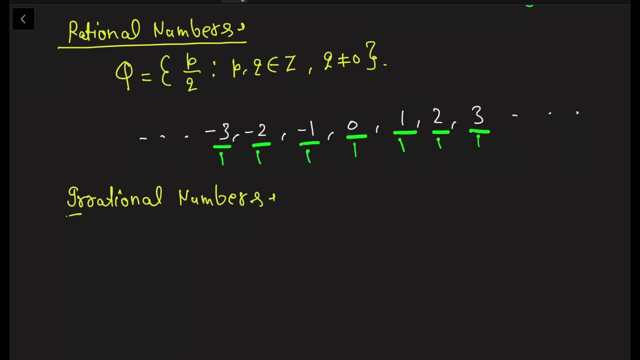 Now, what kind of elements are there in the irrational numbers? What kind of elements are there in the irrational numbers- Let's denote the set of irrational numbers by qi- And what kind of elements are there in them? In this, there are only elements of p upon q type. 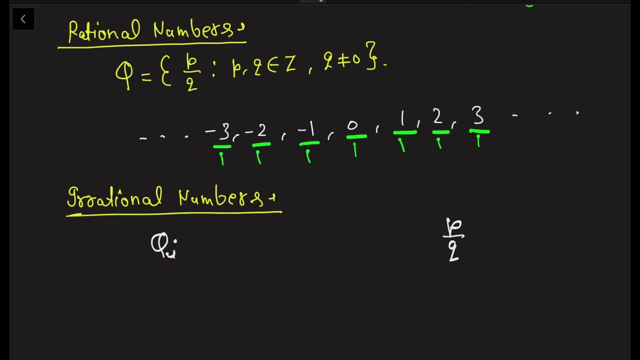 There are only elements of p upon q type in this, But the elements of p upon q type fulfill one condition. only then it will be included in the set of irrational numbers, And that condition is that the decimal number that will come after dividing p by q is non-terminating and non-repeating. 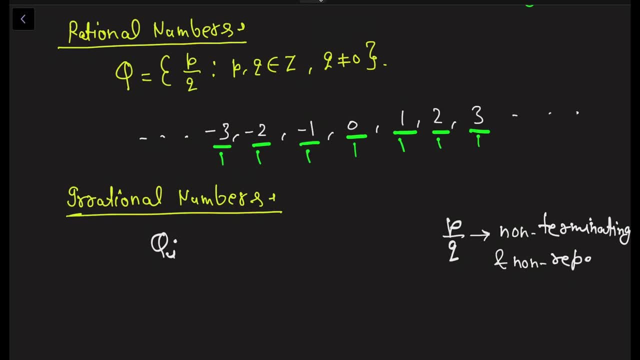 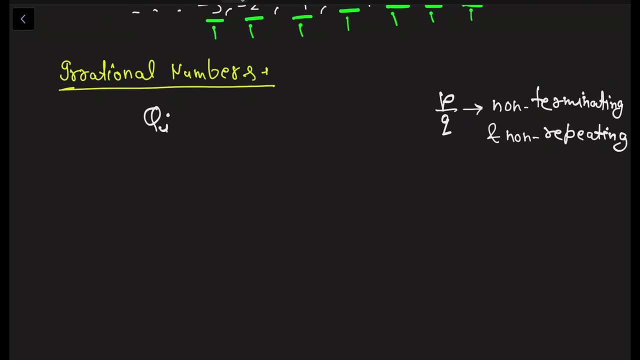 If we satisfy both non-terminating and non-repeating conditions, then the decimal number that satisfies the condition of non-terminating and non-repeating will be our additional number. Let me show you an example of this. You know that the value of pi is 22 divided by 7, which is 22 upon 7.. 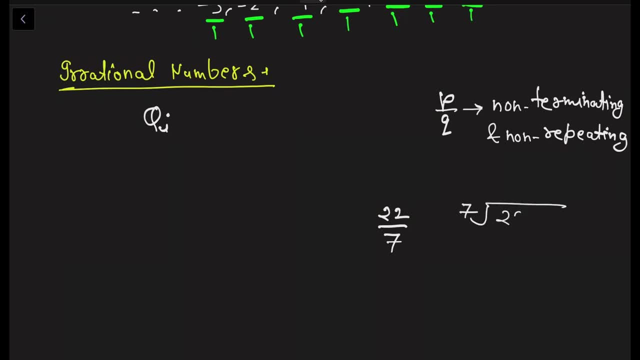 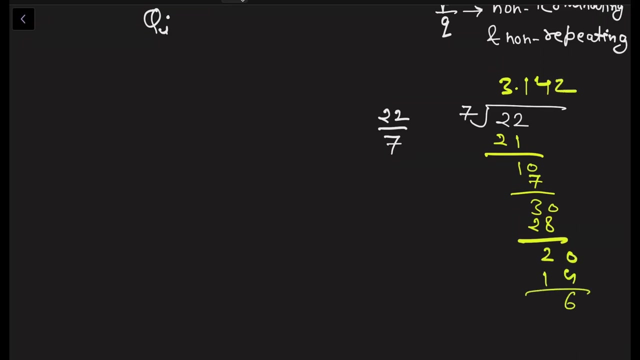 If you divide this 22 by 7. Then 21 will come, 1 will come, 4 will come, 2 will come, 8 will come. Then, after this we can increase it again, 35 will come. 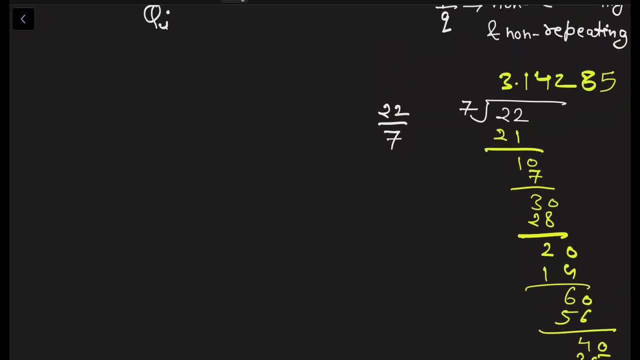 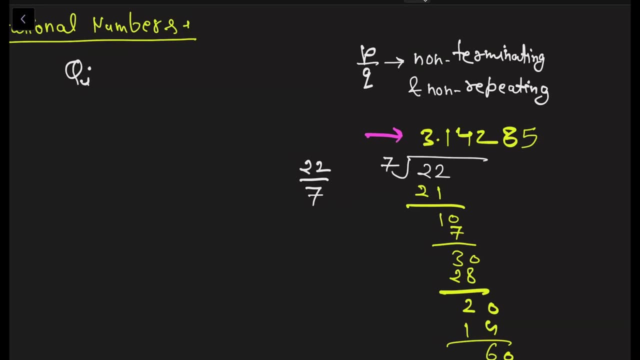 So you can see that we are dividing 22 by 7.. In this a decimal number has formed, This decimal number has formed, And in this the elements that have come after the decimal, the numbers that have come after the decimal. are they being repeated? 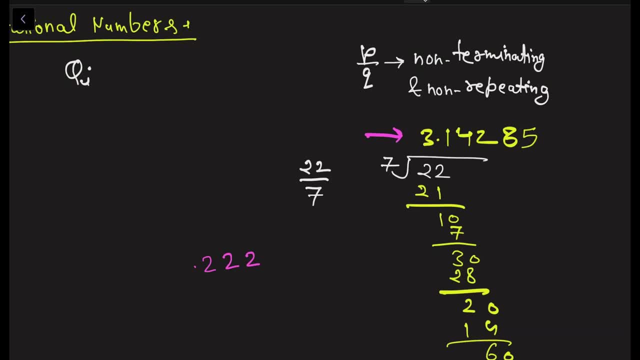 It means that after 2,, 2 came again, 2 came again. Have any such numbers come? No, This means that this decimal number satisfies the condition of non-repeating. Non-terminating means terminating, means to end, And non-terminate means that which is not finished. 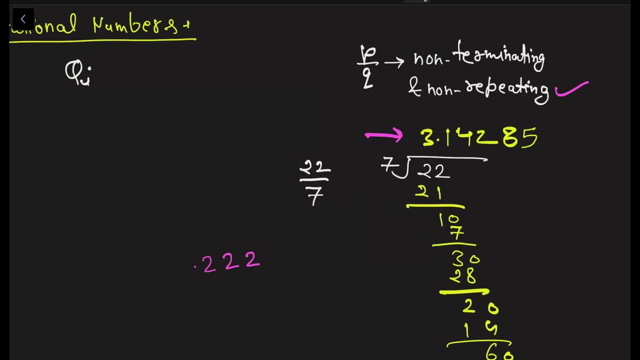 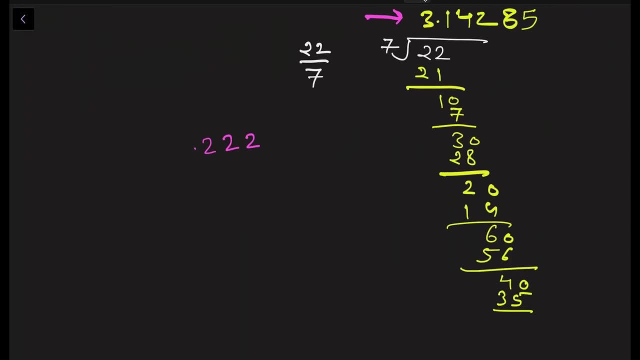 Which does not end anywhere. Terminate means to end And non-terminate means that which does not end. You can see that when we are dividing it, we have reached here And even after this, it will keep going. It will keep going. 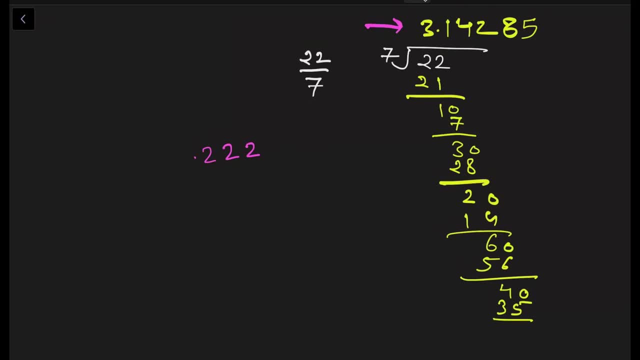 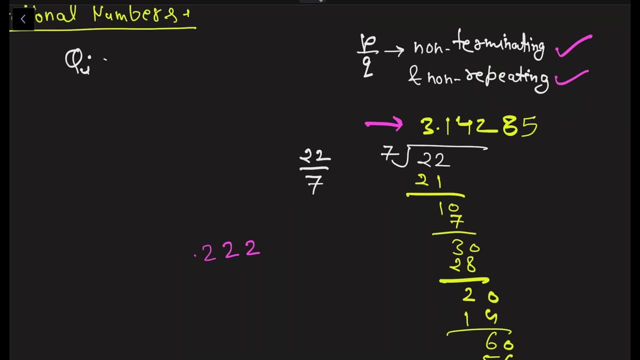 It will not finish anywhere. It will not end, That is, it will not terminate. This means that it also fulfills the condition of non-terminating. That is why our 22 by 7, that is the element that is pi- is an irrational number. 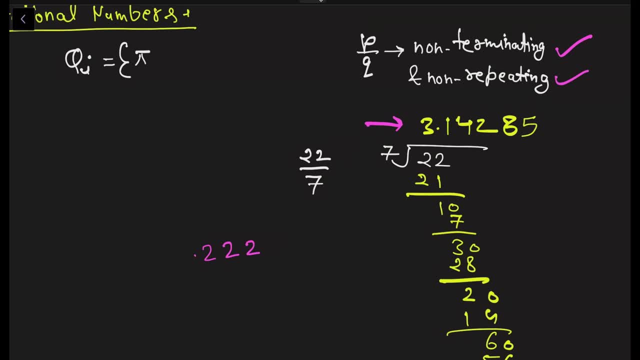 Okay, If it were, it would be in the form of P upon Q. P will be integer, Q will be integer. Q should be non-zero. The condition is the same as that of the rational number above, But what is its condition? 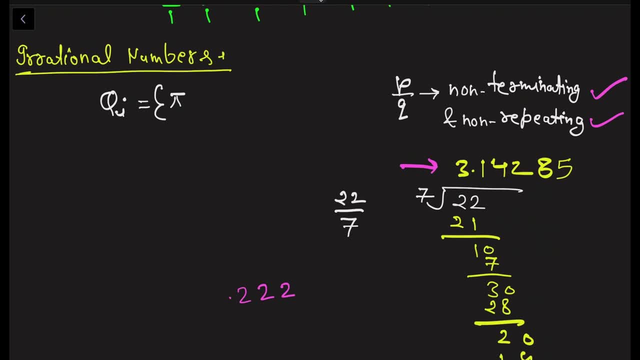 The same decimal number will come in this, which will fulfill the condition of non-terminating, non-repeating, As I told you with an example. Okay, Like pi is done, Root 2 is done. Root 3 is done. 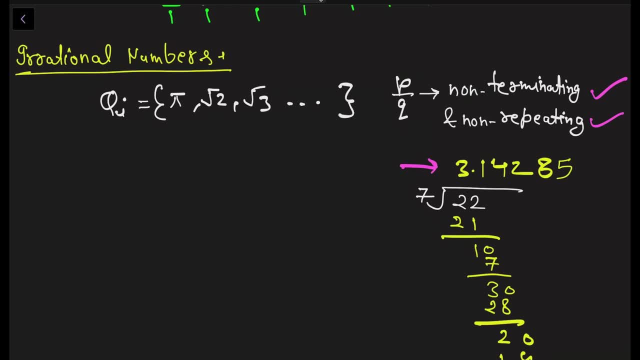 All these are our elements. This is the condition of the irrational number that I told you It fulfills. That is why it is an irrational number And all the P upon Q elements that are different from the irrational number will belong to the set of rational numbers. 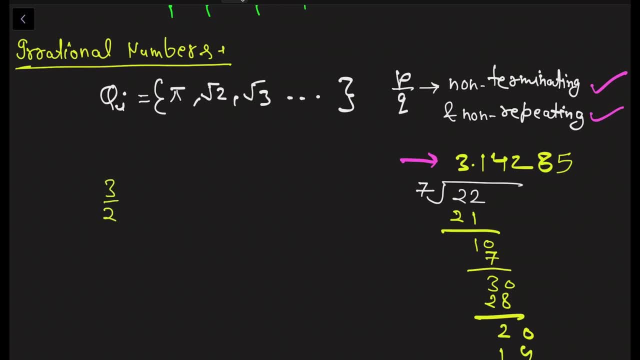 For example. I took one more example. I take 3 upon 2.. If we divide 3 by 2, then 2 will come, And then our pi will come, And then it will come 0.5.. So what do you see from this? 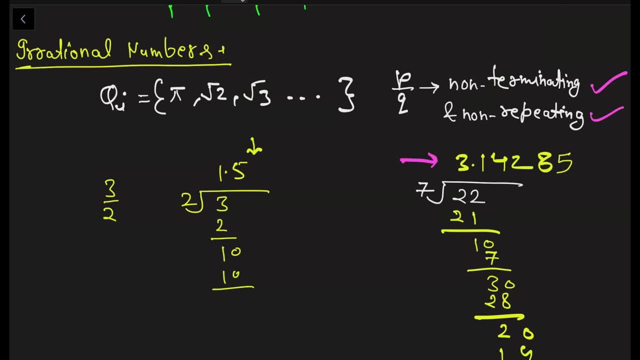 It has been terminated. Terminate means it ended here Once your decimal number came 0.5.. After that it terminates, That is, it does not satisfy the condition of this non-terminating. So in which number will this number belong? 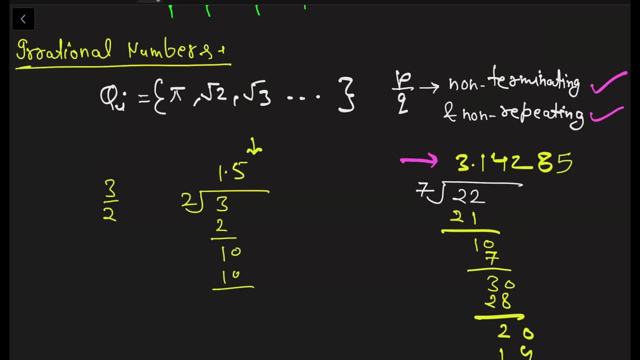 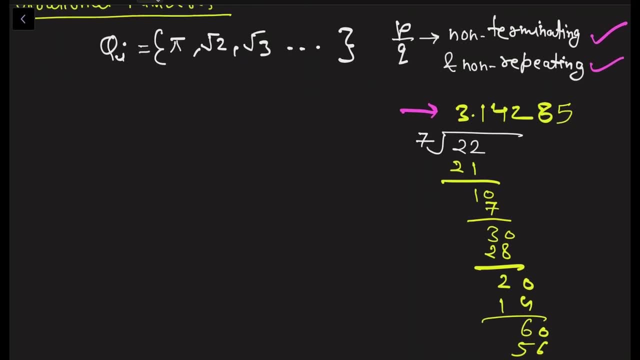 Will belong to the set of rational numbers. Okay, That's what I told you: elements which are non-terminating, non-repeating, if any condition is not satisfied, then it will become a rational number. So these are some of the elements of our rational number. I told you, by definition, how elements belong to it. 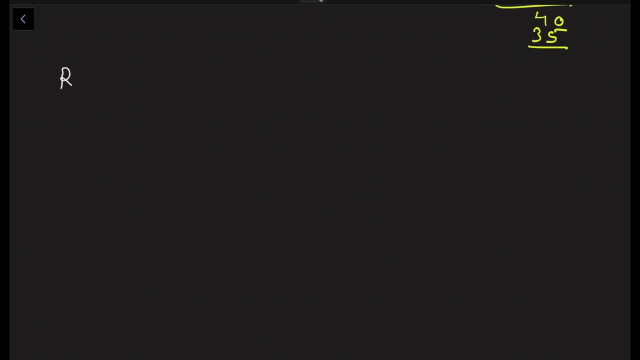 Then we make a set of real numbers. we denote this real number set with capital R. Now, how will the capital R real number set be made? Because I told you that all the integers are also rational numbers. Now, what is a real number? 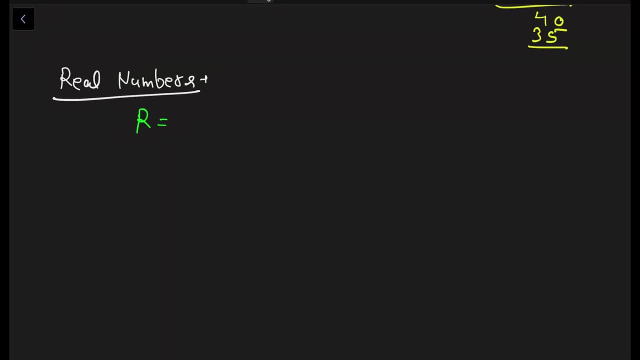 A real number is a set that covers all the elements coming on the real line. That means there is also an integer in it. Rational numbers also come and irrational numbers also come. Simply say that if the union of the set of rational numbers is set with the set of irrational numbers, then our set of real numbers is made. 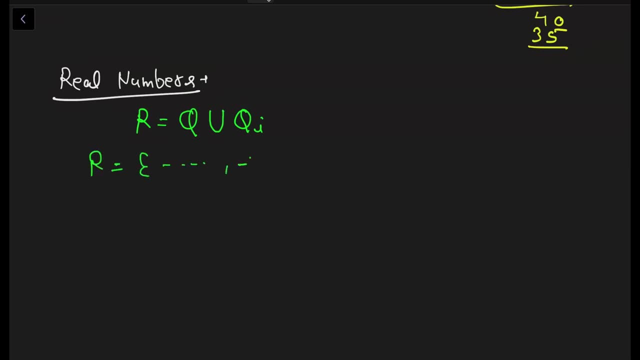 What will be the set of real numbers? It will be such a set that we can write in this way: 1,, 2,, 3,, dot, dot, infinity. In this also we have to eliminate between minus infinity and infinity. 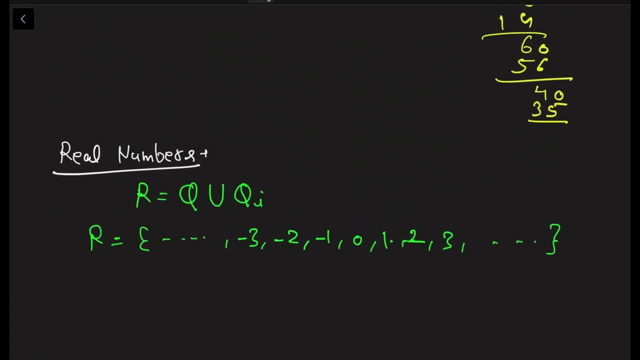 We have to eliminate between minus infinity and infinity. All these elements will be there, But its notation can be seen that it is of the form of an integer. But this has a lot of difference. How is the difference in this? I told you that there is 2 after 1 and 3 after 2 in the integer set. 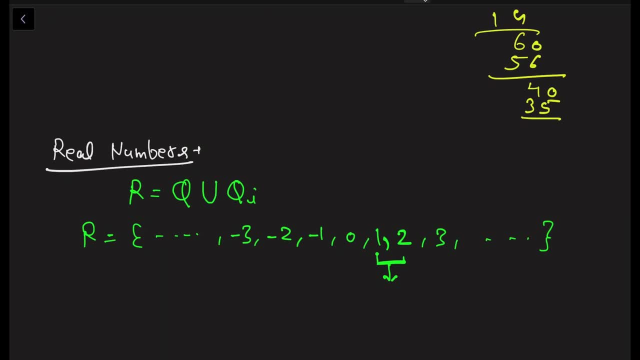 But what will happen here? Infinite elements will belong between 1 and 2.. 1 and 2 will make an interval and infinite elements will belong to it. That means infinite rational and irrational numbers will belong to it. So I have told you the set of real numbers, that is, the set of rational numbers and irrational numbers. if both the sets are collected, then the whole set of real numbers, ie the real line, becomes ours. 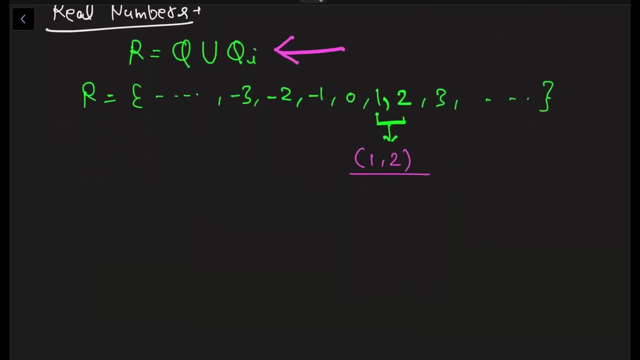 So this is our set of real numbers. Now, a series is formed in this: that the natural number is a subset of the whole number, The whole number is a subset of the integer, The integer is a subset of the rational number, and the rational number is a subset of the real number. 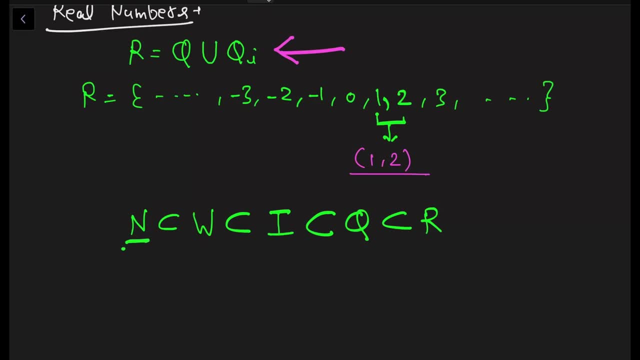 So a chain is formed in it that the smallest set will have a natural number and the largest set will have a real number. Then, after the real number, another set is defined in it, which we call the complex number, Complex numbers. What is a complex number? 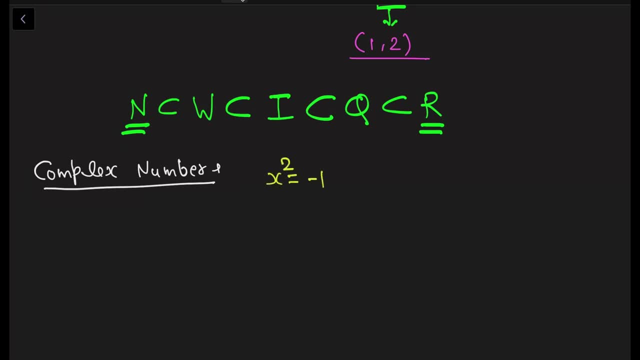 When our condition is formed, we know that x square comes equal to minus 1.. So in that case, in our real case, the value of x will come minus 1 in the under root, which does not define the real. This was denoted by our i, the under root minus 1, and the complex number was made. 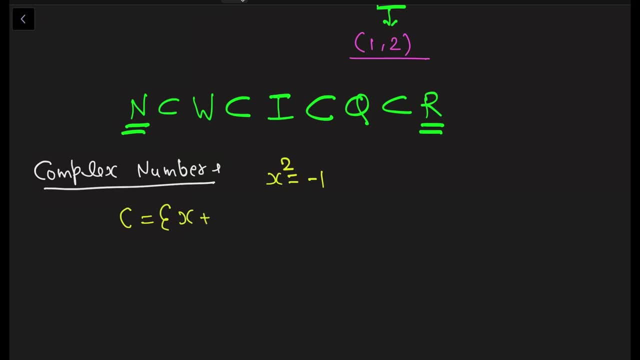 In the complex number we denote from c. In this all the elements of x plus i, y type belong to, where x and y both belong to the real number. Okay, that means you can say that all the real numbers, All the real numbers, are also complex numbers. 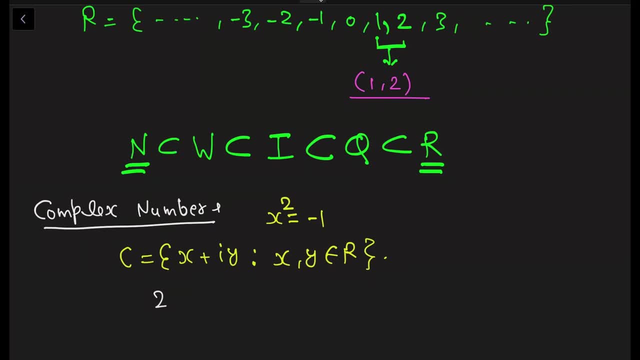 For example, I took 2.. Is it a real number? Will it be a complex number? Absolutely, Because we can write 2 plus i into 0. Which will fulfill this condition. That is all. the real numbers are also our complex numbers. 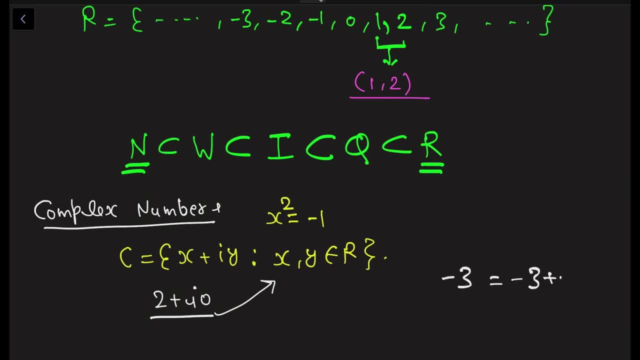 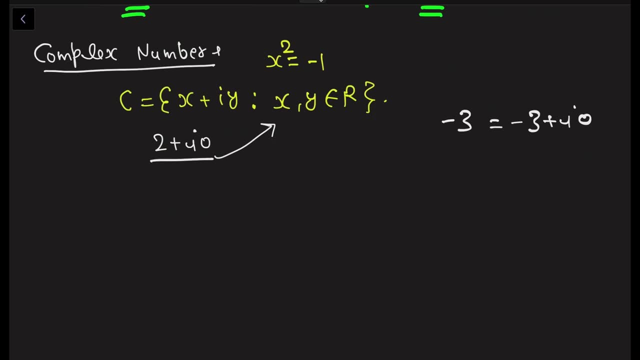 For example, we can write minus 3 plus i into 0. Then it will become a complex number. That means all the real numbers are also complex numbers. Okay, In the end we can say that the whole number will be greater than the natural number.